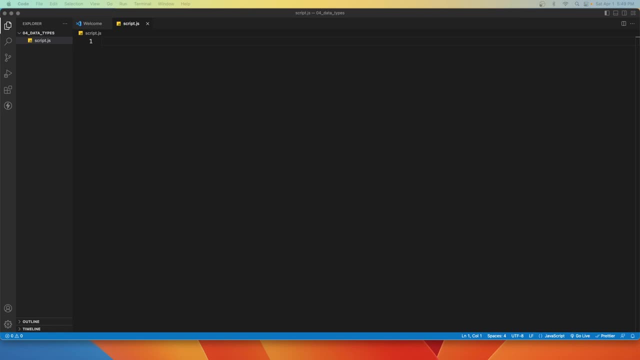 And what you'll notice here is, in the previous video we actually declared some actual variables in which we did something like this: We did let my number equal two. Okay, Now, one thing I may have forgot to mention is we could actually just declare it and use it later and say my 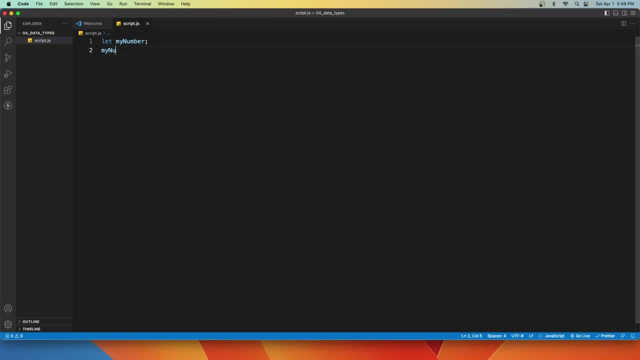 number equals two. We can definitely do that as well, But in this case we're going to use the script file. So let's go ahead and let's start with the number type or the numeric type in which my number is going to equal. 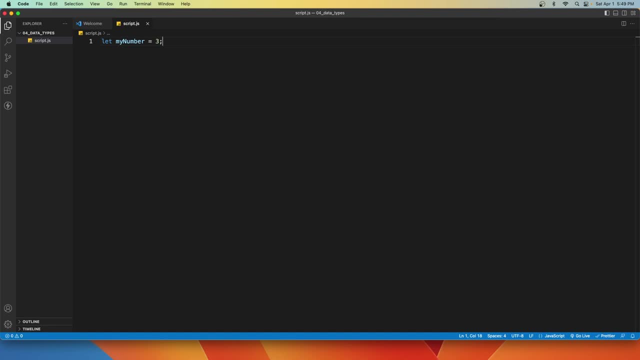 three, And now we can actually utilize that variable for whatever use case. So that is the actual number for the data type. And again, just remember as a review from previously, in different languages like Java or C or C++, you would say something like string name equals. 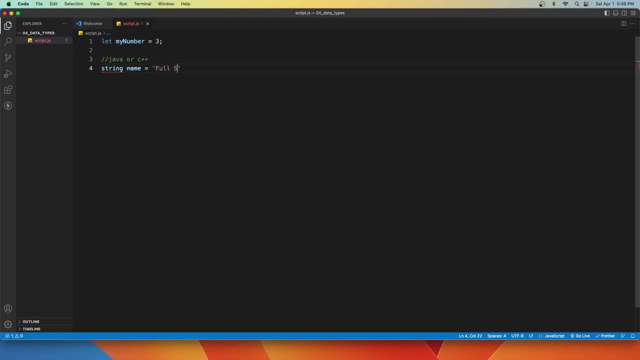 full stack. But we don't have to do that here. No, we don't. All we have to do is just actually assign the actual, not assign the type, but just literally just place it in there. So in this case, we literally just said: number is going to be three and JavaScript. 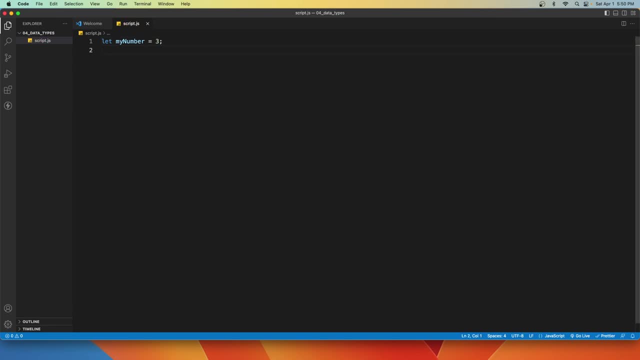 will say: okay, three is a number, So my number is going to be a numeric value. All right, So now let's go with a string. We'll say my string, or actually we'll just go with let name equal Full stack, in which full, full stack is actually a string. So in this case, name is going to 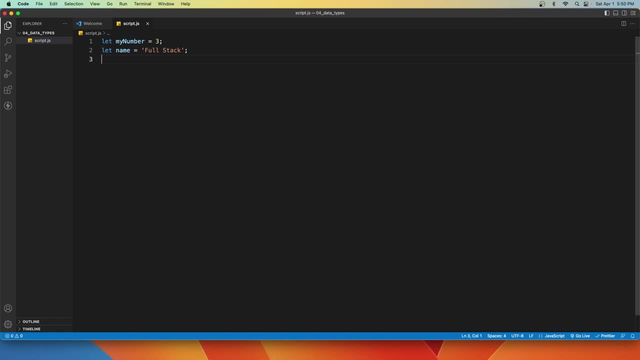 be a string. So that's the numeric value. There is the string value. Let's see what else can we go with. Ah, okay, How about a Boolean value? So that's going to be like a, like a true or false. So in this case we can say: let's say is valid. You know, sometimes 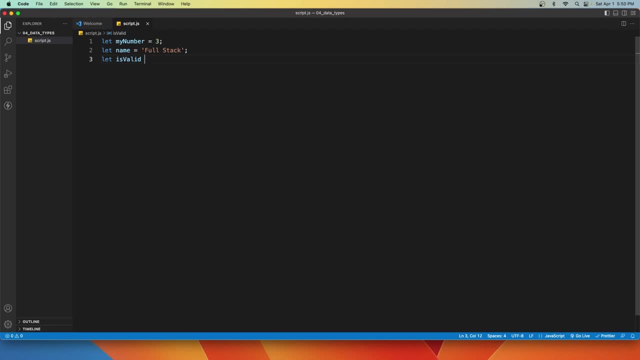 we have things that are either valid or not valid. So let's say, is valid, Is valid, is going to be equal to true. Okay, So that would either be true or false, in which you might have to test whether or not a page or some credentials are valid or not. So we'll. 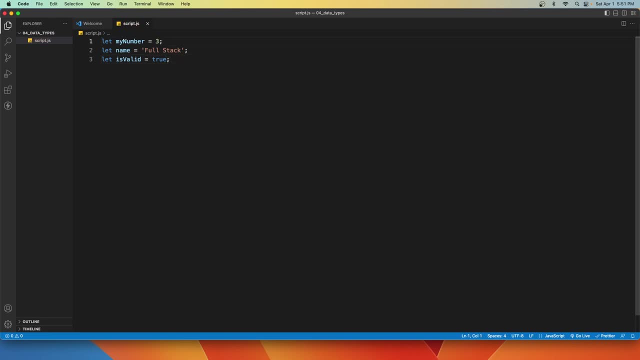 say: this is a Boolean value. So the first one we have is numeric. The second one, which is the name variable, which is given the string full stack, Um, so that is a string and is valid, is a Boolean value in which that is a true or false. 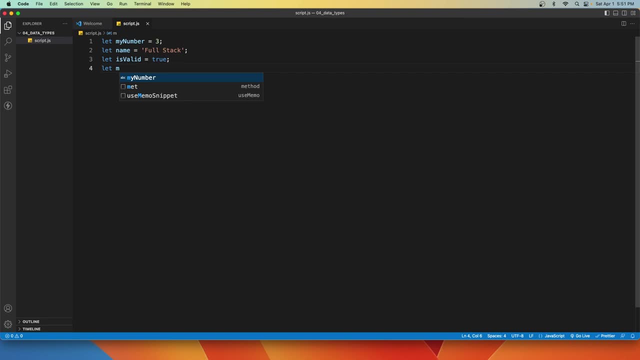 Now we also have the array. So let's just say, um, my array equals uh, and in this case we'll just give it. we can give it some values: one, two, three, All right, And that is your array, very similar to other languages as well. And let's go with an object here. 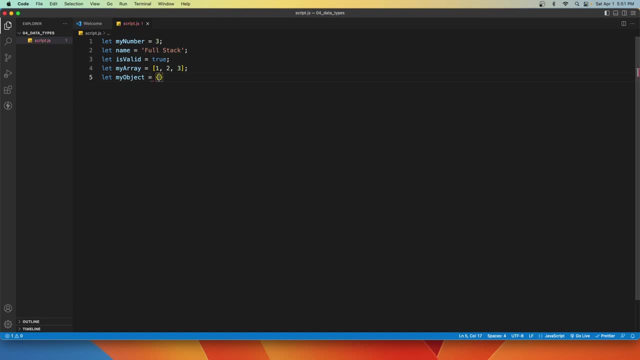 We'll say my object, And in this case we'll open that up and we'll give it some key value. pairs in which we'll say name Actually, we'll bring it out on another line. here We'll say name Actually. how about? 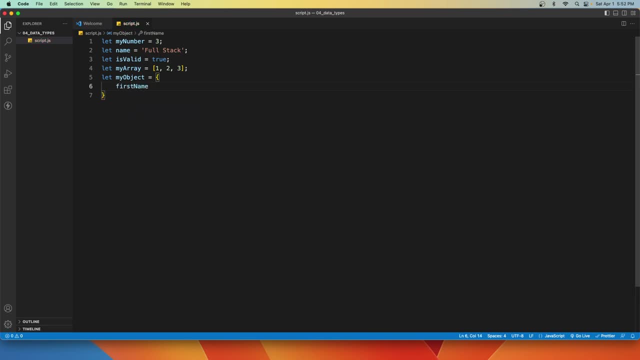 the first name, first name, and we're not going to go equals, but we're going to actually do a colon here And then we'll say that name is going to be a string. We'll say, uh, uh, Mr Blue, Okay, And we'll give a last name of, let's say, um, Mr X, X, nine, Okay, And 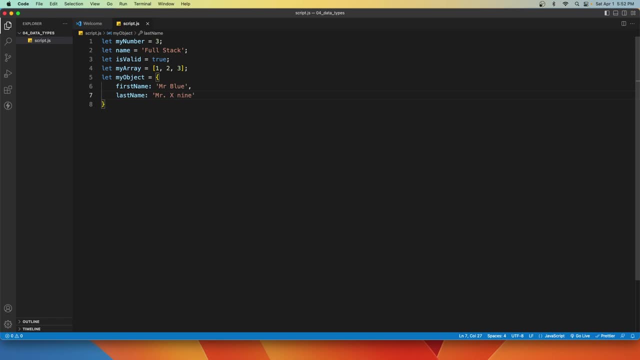 we'll say: uh, X, nine, All right, For lack of better names here. Okay, So there's an object. Um, our objects can have a number of different, uh, a number of different variables and values as well. Um, so we can actually say something like: um, let's say we have. 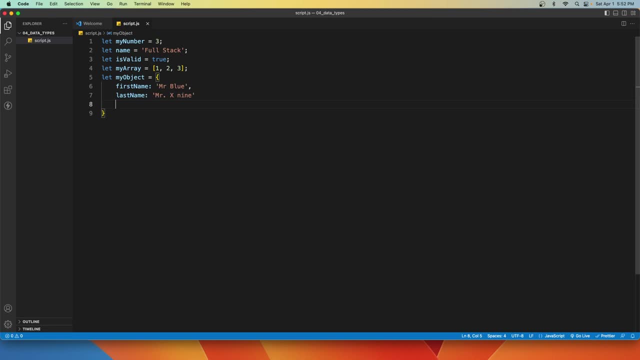 first name, we have a last name. Um, let's say, let's say, if it was a game and he had a power or a number, actually, well we could just say: uh, his array, We'll just say his. 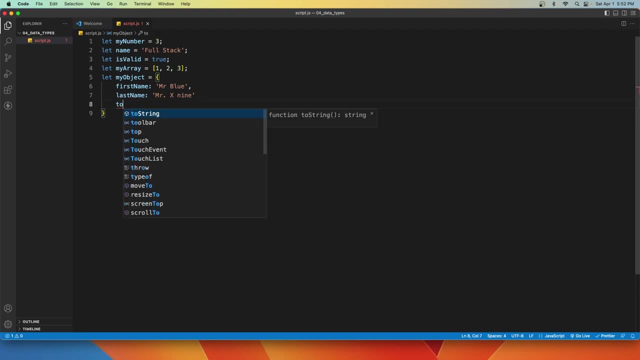 array, or actually his well, let's do. he has, let's say, my object has a to do list inside it, And that to do list itself is an array of, um, let's say clean house, and they'll have another element in there of, uh, let's say clean the garage, Okay, And oh and we. 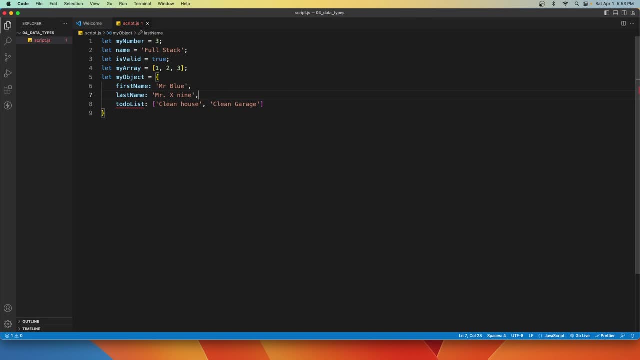 have a little error here. That's because we are missing an actual comma. Okay, So that is the object. So we have a numeric value, We have a string value, We have a Boolean value, We have an array. Uh, we have an object and what else Is there? 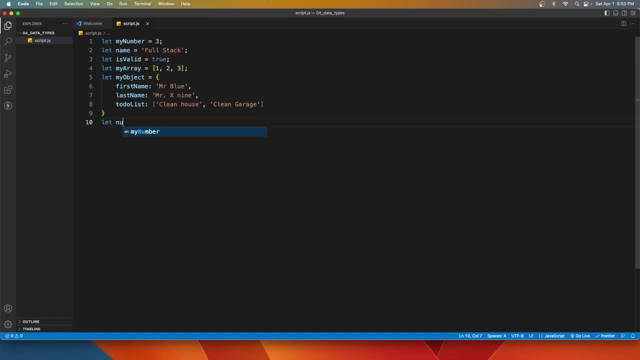 anything else missing. We could say: let something be undefined. Um, let's see, uh, how do we want to? we'll we'll? we'll just say we'll call it undie, undie, let undie, equal, undefined. 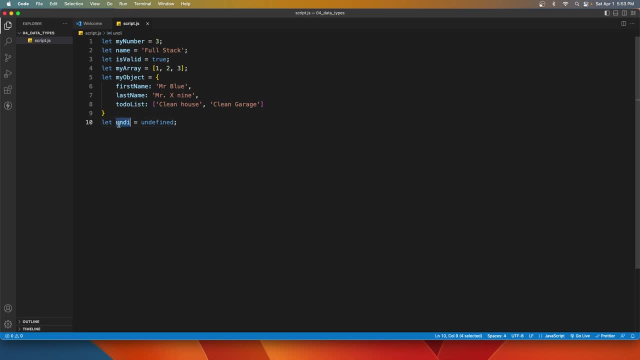 Uh, we can do that. in which. what does this mean? This means the. this is the. it is actually, it's declared. So undie is declared, but, um, it doesn't have an actual, an actual value. So we could actually leave it like this, and it would still just be undefined. 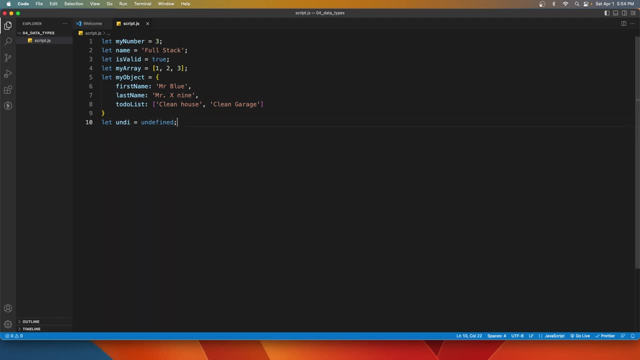 Um, but let's just say, we'll say it's undefined. Uh, actually, let's, let's leave it blank, Let's leave it blank. And I think the other one would be: let null or net null. Let's say, we'll call it my null, which, in this case- this is basically null- is like similar to. 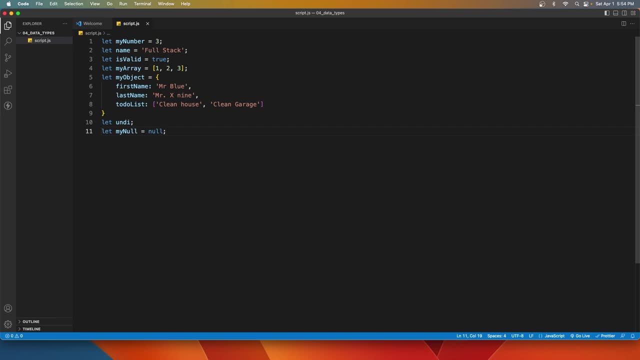 zero, but in this case, um, it's declared and it's just giving it just a null value itself. So these are just the main ones here, Uh, the majority of the ones that we have that you would actually use, Um. so, just to recap, we have the number, we have the string. 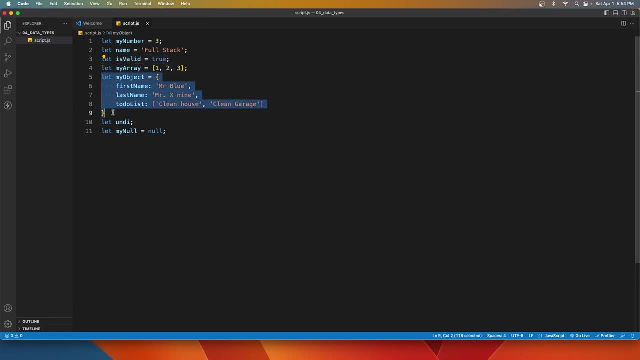 we have the Boolean value, we have the array, we have the object, which could have a number of any of these as well, And we have here. we have something that's actually just declared um, but it has no value, So it is going to be undefined, And actually, you know what? 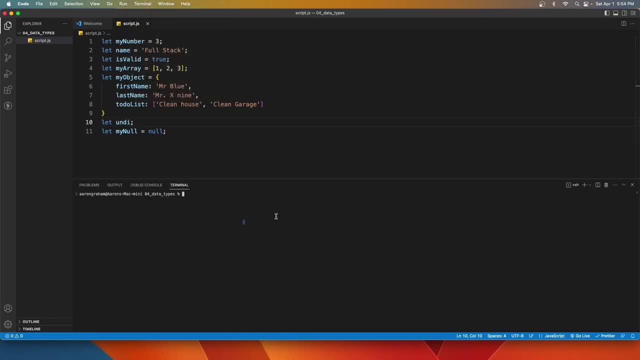 let's just take a look at that in the terminal as well. Let's take a look here. Let's console log: Um, I do want to see, is it? and this is a good little test here. let's console log, undee and see exactly what we get. just want to make sure here and then over. 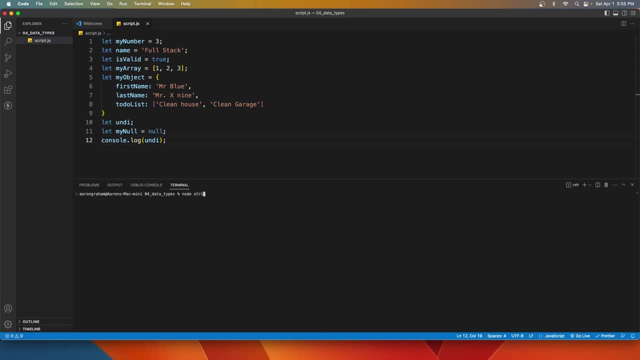 here. we'll just- actually we'll just- run this and it's the name of the script, okay and okay. so we're logging out undee and we actually get undefined, which is definitely good. so that just means again it's declared, but it doesn't have a. 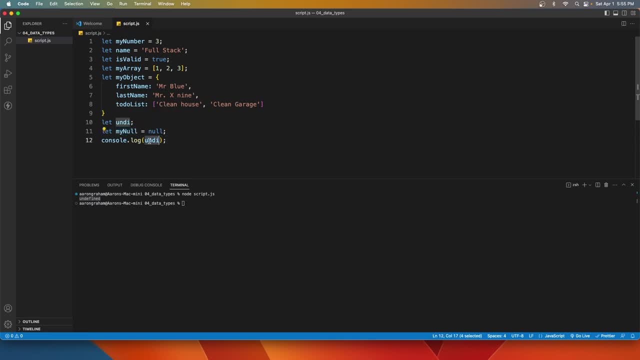 value, and now it's actually logged out my null. let's take a look and see what we get with that, and that comes out as an also. alright, so perfect, perfect. so this is data types in JavaScript. a little bit long there, but you'll definitely be utilizing a number of these. we will actually go into further.